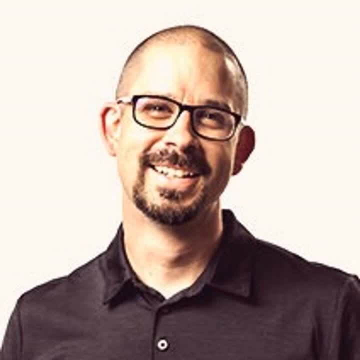 and was more open and was working on open source activities and partnering with other agencies and trying to figure out how to help developers get more active in the open source community from contributions and releasing projects, And so it gave me an opportunity to be a less mysterious. 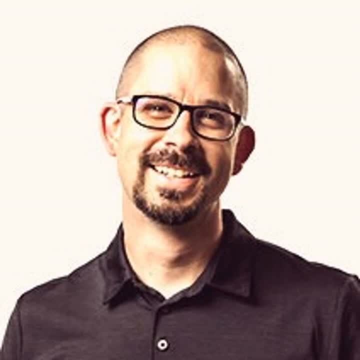 face. on behalf of the agency. Yeah, you were like the senior OSS evangelist and I'm trying to get my head around how you would even pull that off. I mean, I just assumed if you worked for a three-letter acronym agency, then you would just not even tell your neighbors. 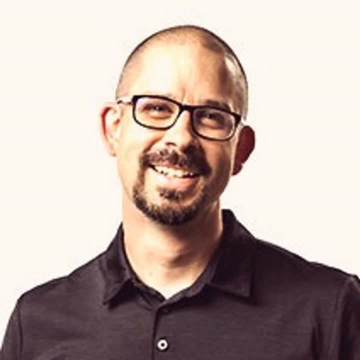 right, Like we see the TV shows. What do you do? I work for the government, That's all I can tell you. But you're like, no, I'm evangelizing. open source for the NSA. How did you connect the two? 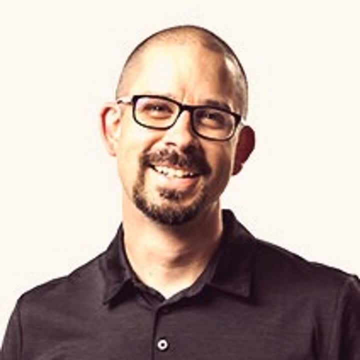 Yeah, I mean, I think it starts, as many of our stories do, of just following a passion, following an interest. We're working on a project and we thought it would be great to open source it because we wanted to partner with universities and the military and other places that didn't. 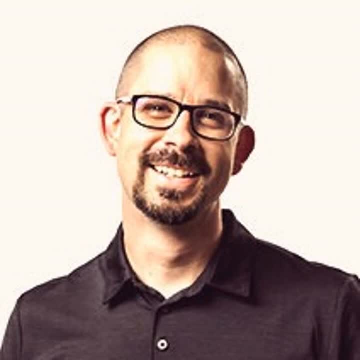 necessarily have access to the open source. So we're like, oh, I'm going to do this. internal networks we were working on And that spun an 18-month effort to release a million lines of code And I learned a lot in that process and wanted to make it better for other developers And 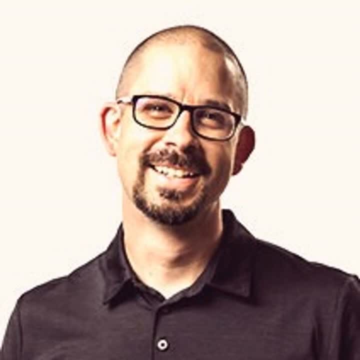 so I really just kind of leaned into that and spent some time looking into it and talking to folks and figuring out how we do more of it. So what's cool about that is that it fits nicely into why you would come to GitHub. You basically became so open and so into open source. 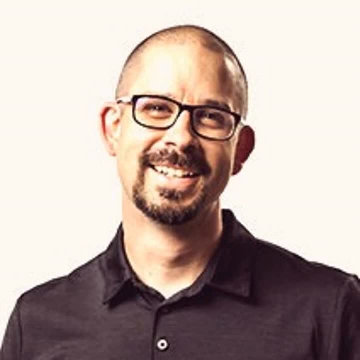 that that passion led you into doing open source at GitHub. Yeah, exactly, I couldn't think of a better place to come after my time in the federal government- And the fun thing is too. in some of the other things that I was involved in at the agency, I really got to understand and think. 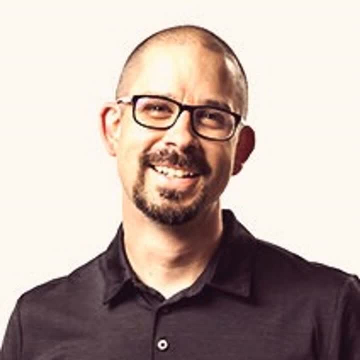 about risk at very high levels, as it may impact nations or critical infrastructure and things like that, And so, combining the leadership training and the risk training, I got at the feet of some very amazing leaders there with my open source passion. working on security at GitHub has been. 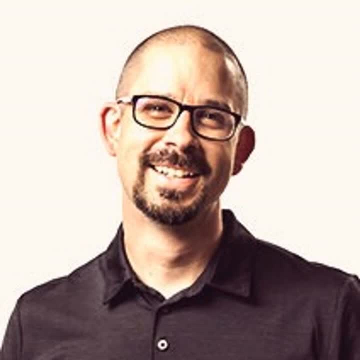 a really great and natural next step for me, And I think actually we may not have met in person, but we were both, I think, at All Things Open in 2020 in North Carolina. Yeah, And you were talking about DevOps. So where does DevOps fit into your life? I know that the name 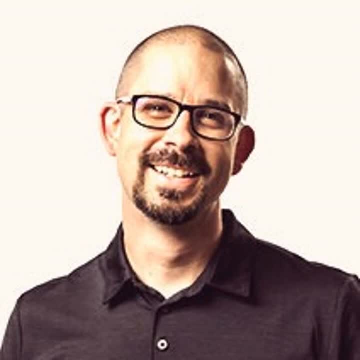 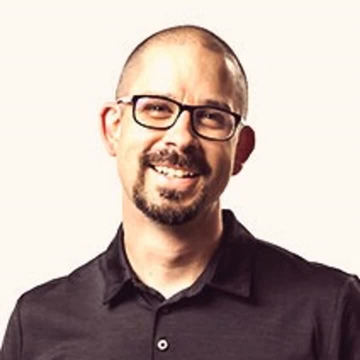 And it became evident that that was only one piece of the puzzle, And so, without a consistent developer experience platform for the developers inside the agency, the open source piece was more difficult to achieve, And so a group of us- actually two or three of us- got together and 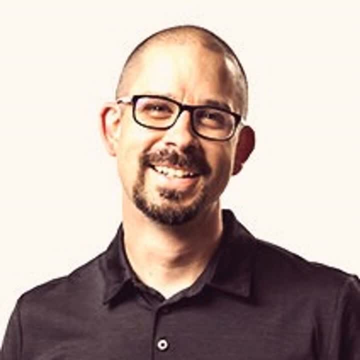 essentially kind of did a startup inside the government. We put a pitch deck together, We got funding, We put all the kind of pros and cons together And we started a program called DevX that ended up Kind of being responsible for all the DevOps pipelines, developer security. 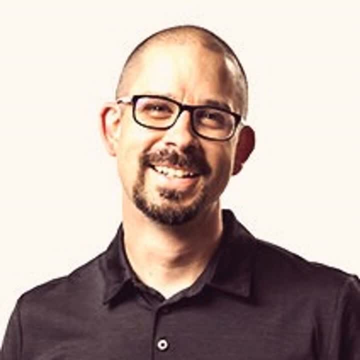 collaboration tools and kind of all the things that you would need to be successful for an agency of 40,000 plus folks. Is it fair to say that even in 2024, there are companies that are just probably building on someone's laptop and then don't have any kind of mature DevOps slash, build server slash even? 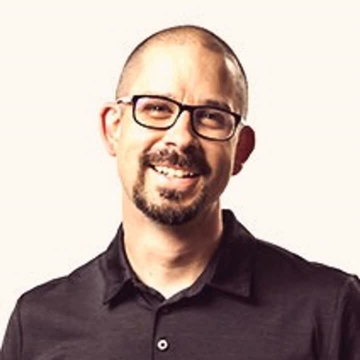 DevSecOps kind of a practice within their organizations. I think that's true. I think we also see a lot of fragmented Approaches where there's 10 or 20 instances of get servers and things are under people's desks and codes spread around enterprises and they're not getting the benefits of sort of the central. 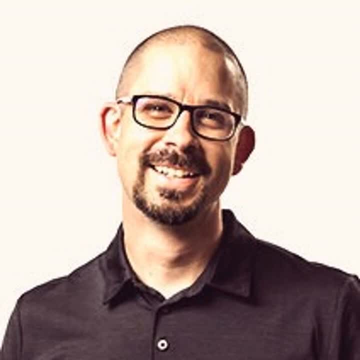 collaboration, tooling and security. honestly, that comes with some of the things that you can do when you pull those things together and take the burden off of individual developers. Yeah, The under someone's desk totally resonates with me. There's so many times. 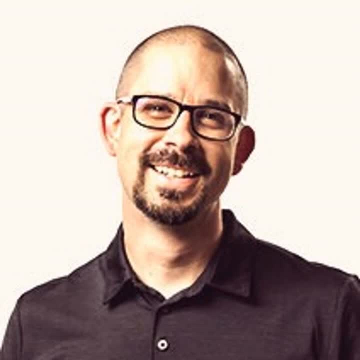 It's a story that I tell a lot, but long story short. my blog, I thought, was a virtual machine for many years And then when it finally died and I called support, it turns out they had never moved it into a VM. It had always been under someone's. 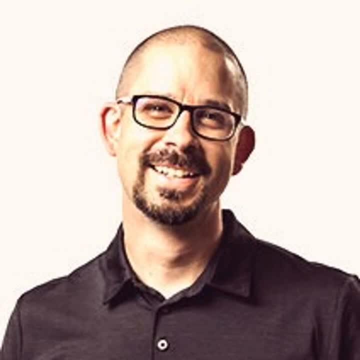 desk. It was literally like a mini tower under someone's desk And they were like, well, we're getting around to it. It was like a hoster service. They never imaged it, They never backed it up. So I FTP'd in, did a frantic backup and the little spinning hard drive finally just 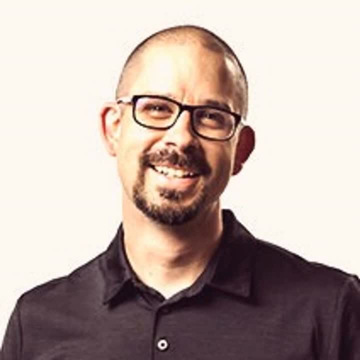 pooped out at the end, But I can visualize it under someone's desk. Never been more More true that the cloud is just someone else's computer, then, But it's someone else's well-run computer, right? And that's the thing I think people don't I. 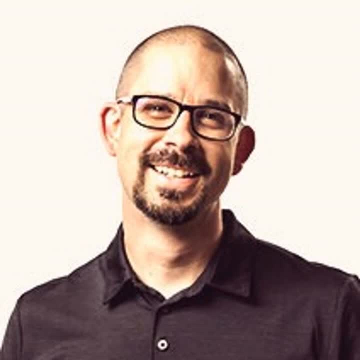 joke about that too. It is someone else's computer, But it's a best practice. It's like we are figuring out those best practices as a community. Yeah, absolutely Absolutely. You mentioned one of the things when you were talking about listing out the pipeline of all. 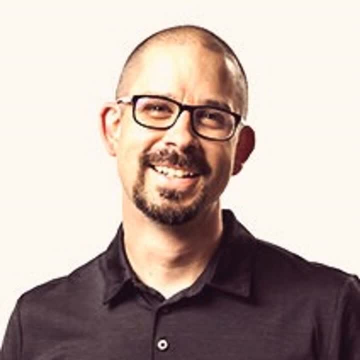 the things For regular Joes and Janes like myself that have maybe a small business like this podcast. I've got the website. I've got to build in GitHub Actions- I keep calling it a build server. My DevOps is effectively. I check it into GitHub and 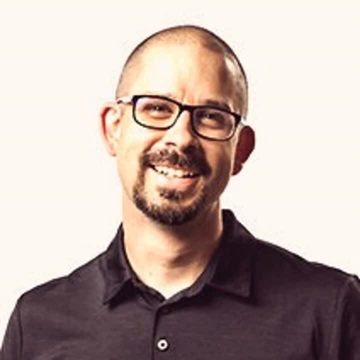 magic pops out the other end. That's kind of as sophisticated as it gets. But you mentioned things like governance and security and the supply chain. Should a regular developer like me, a regular Joe or Jane, be thinking about that level of complexity within their own? 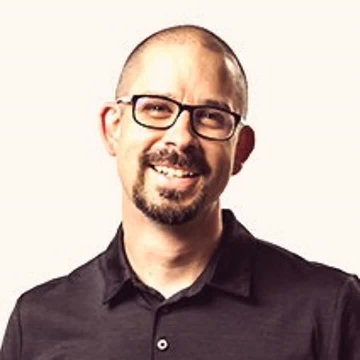 DevOps pipelines. I mean, you're asking the security person this question, so I'm probably going to say yes to some degree. I think the important part here is that it's yes only after the core things are done. So for the fitness folks out there- I've mentioned this before- 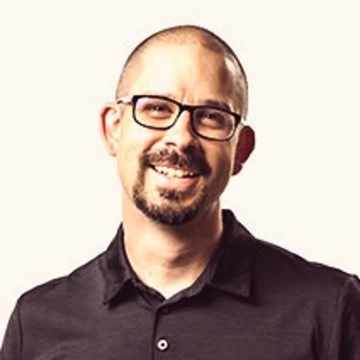 don't ever skip leg day. I think for me that kind of core thing in the security translation is things like 2FA is making sure the account is secure, making sure that things like we don't have storage accounts that are open to the internet and things like that, And I think 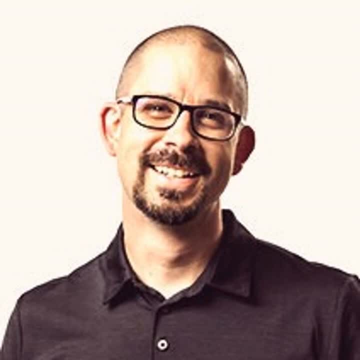 once all those things are done for the average developer, then, leaning into some of the capabilities that, for instance, on GitHub, a lot of our GitHub advanced security systems, security capabilities like Dependabot and code scanning and secret detection are all available for free for public repos, And so I think those are things that folks should. 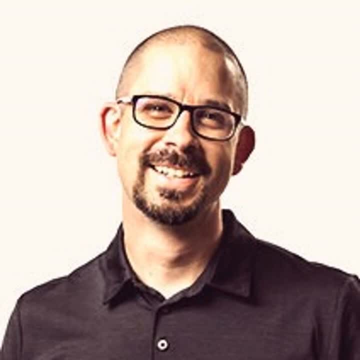 turn on. But for us, when we think about security kind of for the product and for the community, we always start with a developer account. And that's why over the last 18 months or so we've kind of worked through a campaign to turn on 2FA for all the contributors on GitHub, which was a huge effort, to basically say like: no, this isn't optional anymore. If you're contributing actively on GitHub, you have to turn on 2FA, And that's why- because we just see too many things start with password spraying or a breach. 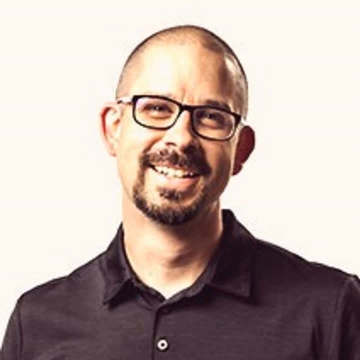 or a credential leak. Yeah, I'm 100% all in on 2FA And I use things like Authy, But then I worry it's becoming centralized Like Authy just, for example, is pulling their desktop app, which makes sense. 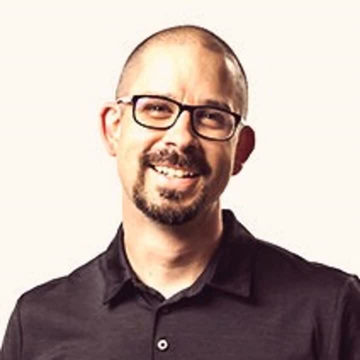 I probably shouldn't be 2FA-ing with the thing that I have in front of me. I should have another factor, But I'm just like: oh man, are they just going to stop caring about that? There's all these authenticator products. 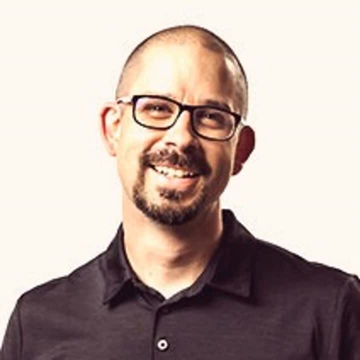 And then, of course, the sheet that we're supposed to print out that no one prints out of their backup tokens. I'm sure that there's a lot of really freaked out people who will lose access to stuff at GitHub if they don't print out their backup keys. 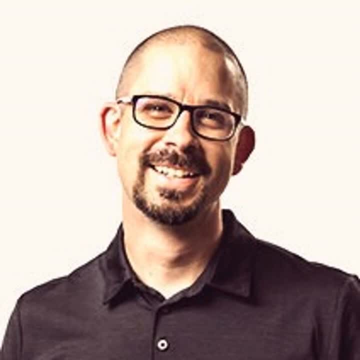 Yeah, I think this is where I'm excited about passkeys and some of the innovations that are happening there, where some of the major companies- and we were actually involved to a certain degree in some of the passkey establishment- are getting together to pull the standardized 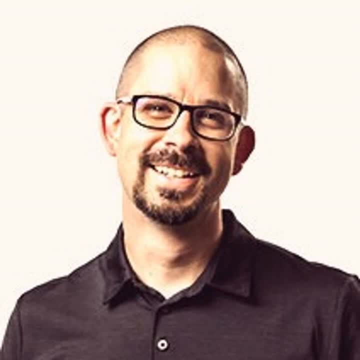 way of doing this together, And you could argue that there's maybe more secure ways like YubiKeys and Biometric And things like that. But as a step forward from username passwords and particularly when it can be stored in a centralized way that's secure, I think it's a great progression that we're excited. about at GitHub. Yeah, you mentioned YubiKeys and I'm sitting here and I'm holding up my GitHub YubiKey that was mailed to me that I never really used because it didn't fit into my lifestyle. And I know that there are people who are so excited about that level, that kind of security, but it just never. 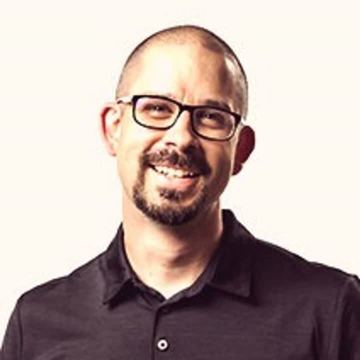 worked for me. Then there was USB ANC. One of them said: and I just got tired. And now it sits here unused, which means that I'm somehow a bad security person now? No, definitely not. I think my YubiKey is sitting in my bag somewhere because I've got all the 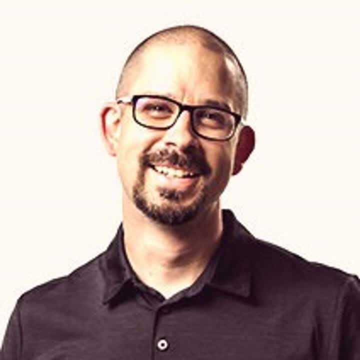 passkeys turned on and FIDO and Touch ID, And so that's how I operate every day. So same security, just don't have to find my YubiKey, And that's the thing, right? Security has to fit into our lifestyles, right, If it is. 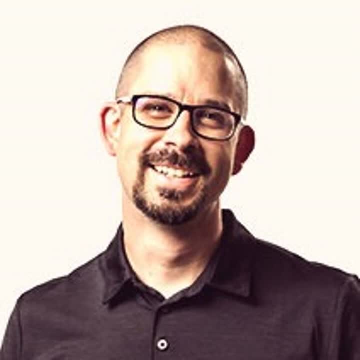 inconvenient enough, then we're just not going to use it at all. Yeah, that's right. We have to make it work for users And that's partly why, even though we're requiring 2FA for contributors on GitHub, we're not requiring YubiKeys or passkeys or anything like that, because the diversity. 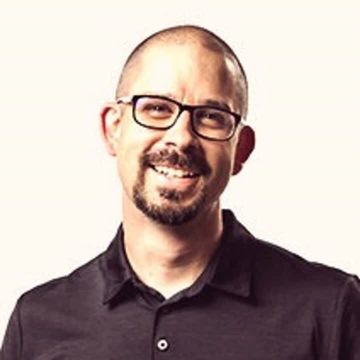 of the population that uses GitHub for open source is huge, And not everybody has access to a mobile phone or modern tech and can afford things like that, And so we want to balance security here with the accessibility and equitability for our user base. 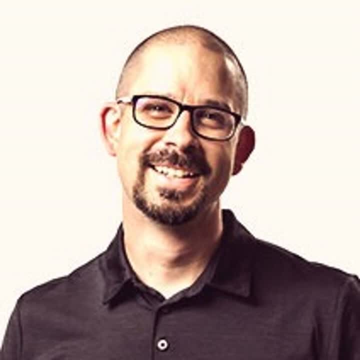 Yeah, I appreciate that You call that out. by the way, like equitability, like even the pricing is modest. You know GitHub Pro is like four bucks And you know for a time there before private repositories were free, it was like seven bucks. I mean it's not big money to support your small. 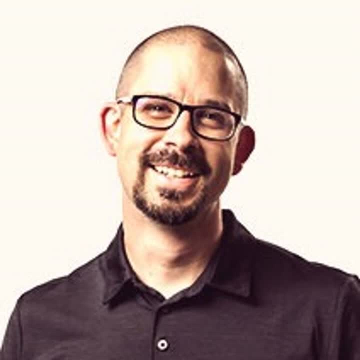 projects. Yeah, agreed, And I think you know we're still one of the few larger SaaS providers in this realm that offer free compute as well. So free actions, minutes and free code spaces, minutes and things like that, And particularly for universities they get an even, you know. 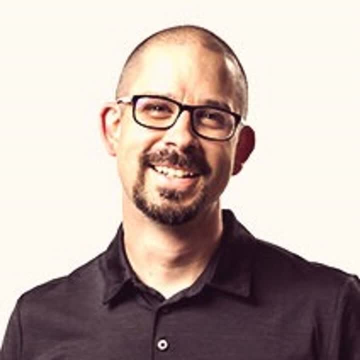 more attractive kind of onboarding package there, which is intentional. right, We want to support the educational use cases, but it's great. It's a great way to get started. Isn't that attractive to bad guys, though? Like the second, you say free compute. 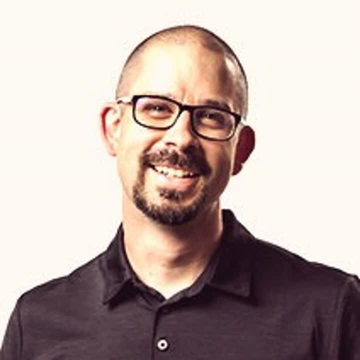 then someone's going to go and start mining Bitcoin or doing something naughty And as an organization that is a giant CMS, you're not only shipping binaries but you're potentially building binaries that could be evil and then helping distribute them. Are people abusing releases? Are people abusing raw dot, whatever GitHub CDN and using it, And 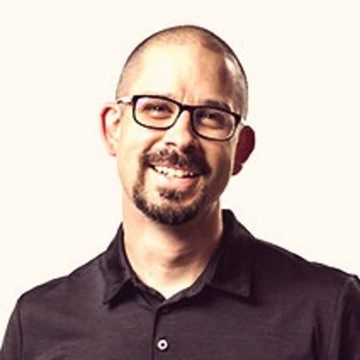 are you constantly just slapping people down? Yeah, it's actually a huge, huge challenge for the platform. With 100 million developers using the platform and a massive amount of compute, there is a lot of folks who are trying to use this for various purposes. So we have in the security team- actually inside GitHub, we have 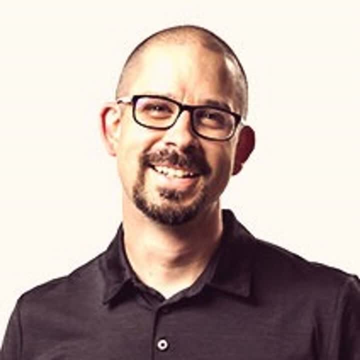 a counter abuse team and they are building machine learning pipelines, auto detections. they're working very closely with support and trust and safety. So as much as possible automate, remediate and kind of shut down Both spam and abuse, but also things like, you know, crypto mining and also things like 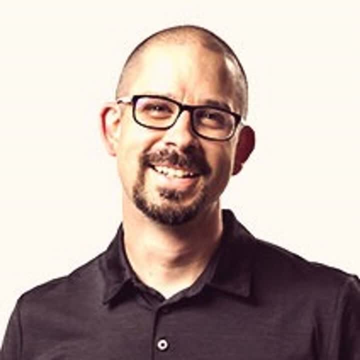 hosting binaries or content that don't meet our terms of service. Yeah, it's definitely a challenging both engineering and scale problem across the board. So GitHub Advanced Security is a product or a collection of products. It's the name for. looks like you've got a friend there in the background. I can hear. 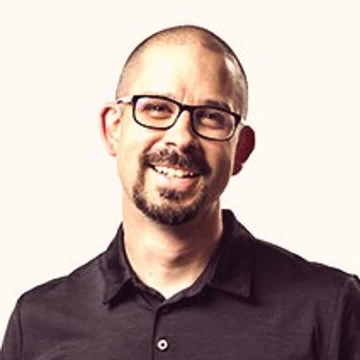 I do Sorry about that. No, it's fine. That's the kind of security that we're looking for, though, at the company, And then someone you'll I assume that there's a bark that you'll hear. That is the I need to get. 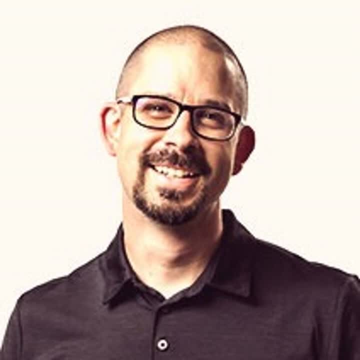 up bark because there's a bad guy, versus the. I see a squirrel bark. Unfortunately, they're exactly the same. Also, friend, bark is the exact same, So that's not not effective as a security tool. You may, We have my. I don't have a dog, but my niece does. Absolutely useless as a security. 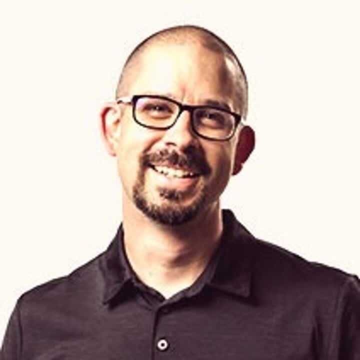 Oh, she's like: Oh, it'll warn me. if no, it won't. No, it will let them in and introduce and it like: bring them over. you know, You see those tick tocks with, like the giant German shepherd, And then like the delivery guy. 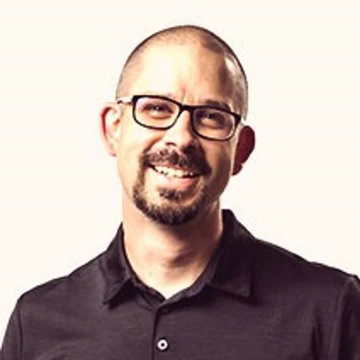 comes in and like, Oh, you do it. Yeah, indeed, That is exactly my dog. I was gonna ask about GitHub Advanced Security and understand, like, is it a product? Is it a collection of products? So GitHub Advanced Security is a couple things, So one for kind of our enterprise customers. 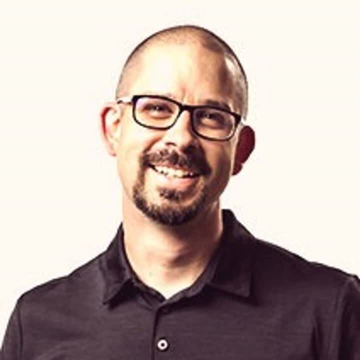 it's a product that can be purchased. that includes code scanning, which is our SAS capability based on code QL. It includes kind of our supply chain Capabilities, which is largely kind of depend a bot and dependency scanning and then secret scanning, which includes push protection. We just recently announced that this is all being 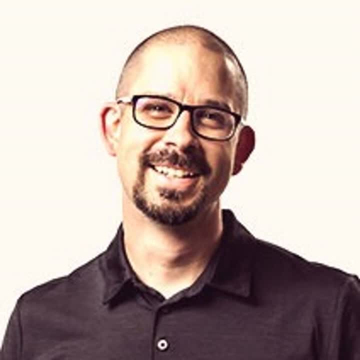 augmented by AI as well. So code scanning now comes with things like autofix, So suggestions. So instead of just like highlighting the potential vulnerability in the code and saying, Hey, developer, you should remediate this, It's coming with an actual suggestion in the pull request to: 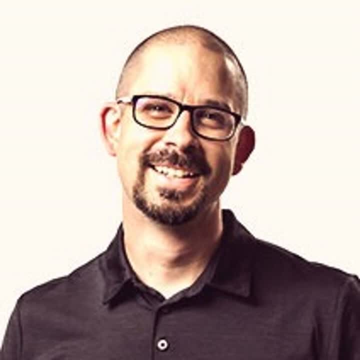 say like: Oh, and here's how we think you should remediate this. you can just click accept and move on from there. And then in the secret scanning space, we're using AI to not just detect high confidence patterns, which is kind of where we've been. 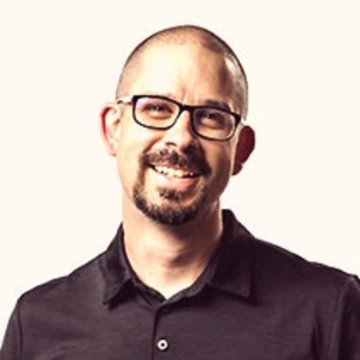 to date. you know things like Azure tokens or AWS tokens or things like that, but also lower confidence patterns like username and passwords or SSH keys or RSA keys. So that's kind of the full kind of GitHub Advanced Security package. Most of that is also available for free on public repos. 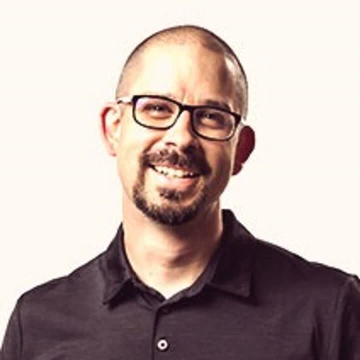 on GitHub, You know- and I have to admit I have abused all of those things- Like if there's a free thing on a public repo, I turn it on and like depend a bot. I could just gush, I could do a whole show on depend a bot. you know, people don't realize how. 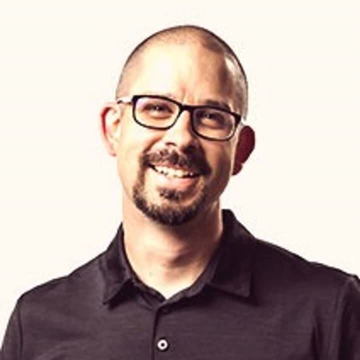 good it is because it's not on by default. right, You get the vulnerability dependencies on by default, But if you're an admin on a public repository, you just go and you check and you turn it on And then you get depend a bot And it's like an employee that makes pull requests. 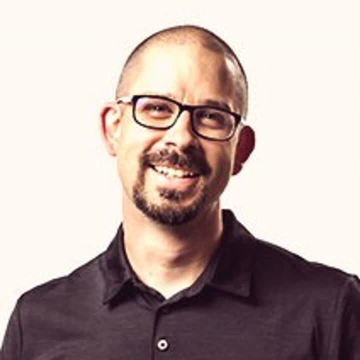 while you sleep, And it's, it's amazing. I gush about how awesome depend a bot is. Yeah, it's really fantastic. And then we're seeing just a huge. I mean secret scannings and newer capabilities For us, but that combined with push protection, we're just seeing some incredible things. 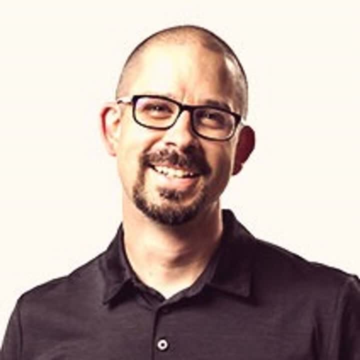 happening. I mean, I'll just give you an example: inside of GitHub we've really worked to, you know, reduce and eliminate secrets in code and our own code base using GitHub Advanced Security and being able to keep it eliminated with push protection so that nothing's getting in there. 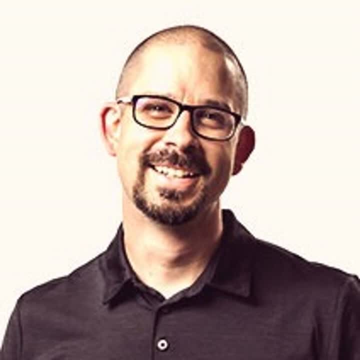 after we've cleaned everything up is just an absolutely amazing capability. But you know, being able to offer that for public repos is critical because you know it's not a cheap thing for us to do from an infrastructure perspective but it's the right thing to do, because we take that responsibility kind of at the center of 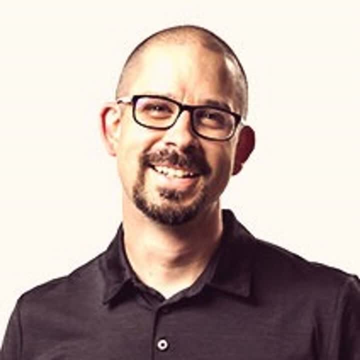 a lot of the software development ecosystem very seriously. Yeah, And this push protection. we should explain that a little bit because, like one of the number one questions on Stack Overflow, like the top questions, is: I pushed a secret into GitHub, I pushed a connection string. how do I make it go away? 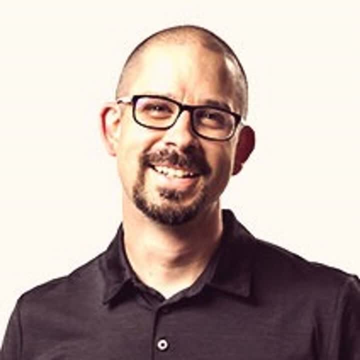 Yeah, I mean that's also one of the number one questions we talk to customers about a lot as well, because it's once it's in, it's in right, It's super expensive to remediate And it's super difficult to know it's good. And if you talk to any security team, they're going to say: 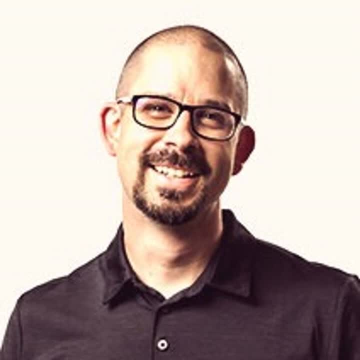 well, like once it's there you got to, you have to deactivate it, you have to roll it, you got to change the credential, And so push protection basically sits in between the editor and the GitHub service itself and inspects. you know it's secure, it's encrypted, but 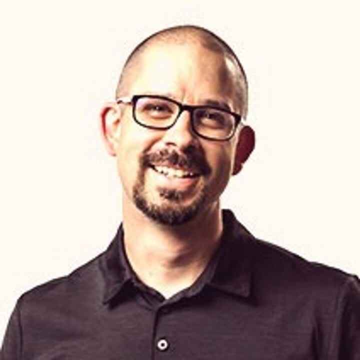 it inspects what's coming in, looking for credential secrets in the code before it actually goes into the get system itself, And if it finds anything, it'll block it. And then there's options depending on you know what's going on in the system. And then there's options depending on 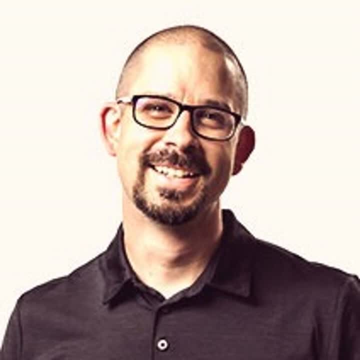 what you're doing. you can come back to the developer and say, do you want to override this? Or, you know, enterprises have the ability to adjust some of their responses there as well, So it's a pretty powerful tool. Yeah, And it really this, this idea of these, these SaaS, these shared access, security tokens. 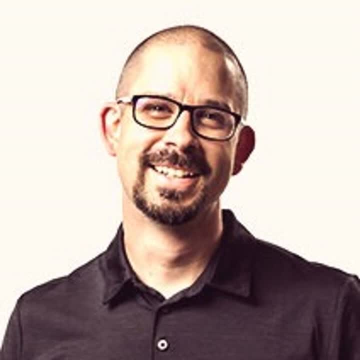 and their potential vulnerabilities. it's just, it's a magic number And if somebody gets it, they own you, And the amount of like responsibility that can be assigned to one of these tokens that is just easily copy pasted and given to someone is huge And I understand. 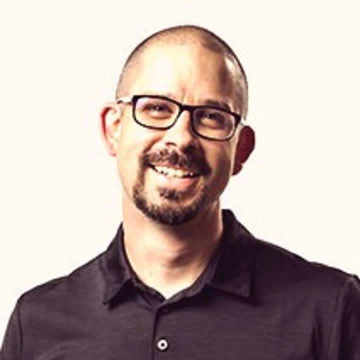 I saw some stuff because I work at Microsoft in my day job. This is all public. There was some nation state actor that got a hold of some tokens and was running around on some you know non-production build servers recently And it all starts with those freaking tokens that you could. 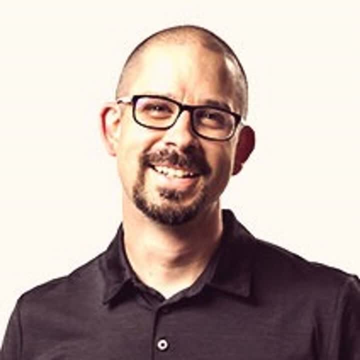 paste to someone in a Slack, So you wouldn't want to catch those. So it makes me wonder, though, as devs, how can we have them without ever seeing them? Like, I don't want it in my clipboard, Because once it gets into my clipboard, it could be given, it could be moved away. 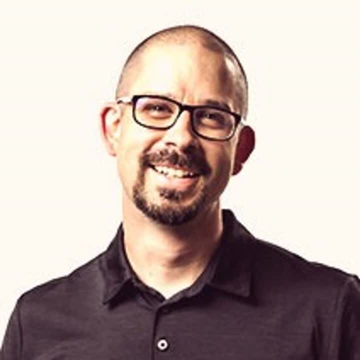 Is there a way to have secrets that we simply can't see? That wouldn't even show up in GitHub? It's a great question, You know, and I think, when I think about the proactive security space and kind of all the advances that are happening. I think this is an area that a lot of enterprises work towards through things like enterprise vaults and kind of accessing these secrets on demand through APIs, which is probably that's one of the right ways to do it. I won't say it's the only right way to do it, but you know, having that 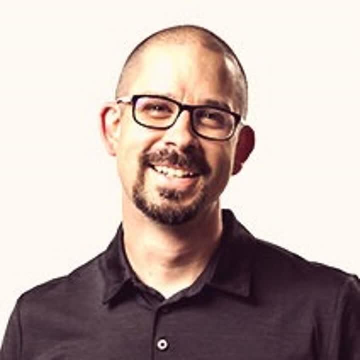 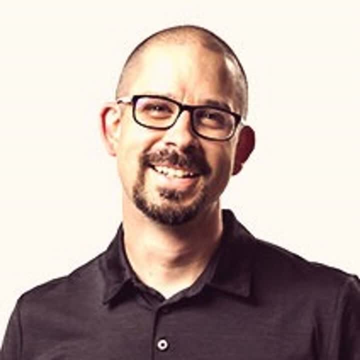 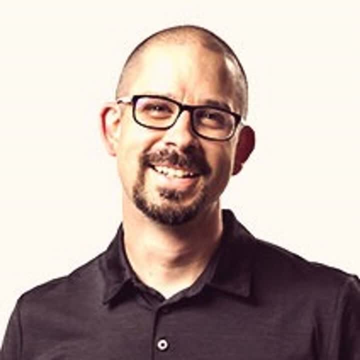 where normalizing things like secret scanning and normalizing and making it clear where to put secrets in places like GitHub or, you know, cloud compute like Azure is helping, but we can still do more, I think, as a community here. Yeah, I like the call out of like normalizing it, Like. 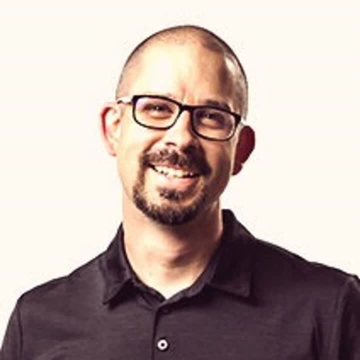 right now, when I start a new project, it usually ends up in some JSON file and that's just wrong. It should be. it's wrong By default And it should be right by default, And I need to like get that into my head so that 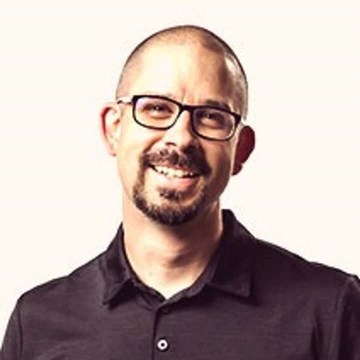 it is normal, And, of course, GitHub will catch me 99.9% of the time or, as you said, it'll warn you and say: are you sure you want to do this? This, this token's used for testing, but even then I 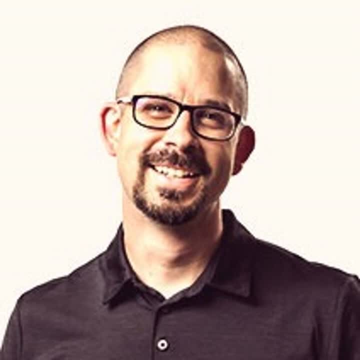 shouldn't push it through. I should do it correctly from from the beginning. Yeah, Agreed, And you know for like that normal dev out there, at a minimum storing it as part of the secret management capability inside GitHub is a good first step, I think, once you start to scale. 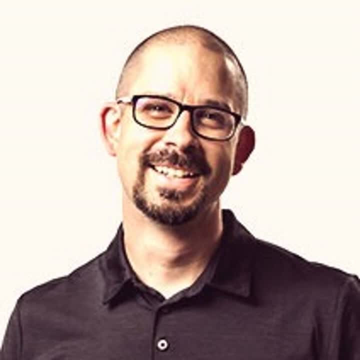 there's probably more sophisticated ways to share that across an enterprise team. So I want to also talk about the third leg of that stool. And we talked about secret scanning, independent bot, but then CodeQL- it's this code analysis tool. It'll analyze your code, It'll give 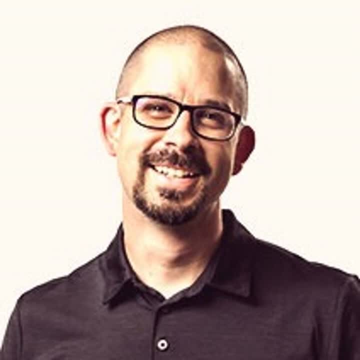 you quality, but it's really becoming a security tool. Like it's spotting like bad practices. but you have to do this across a plurality of languages, right, Like there's all kinds of you know, you could be doing Erlang, you could be doing Rust, you could be doing C-sharp. 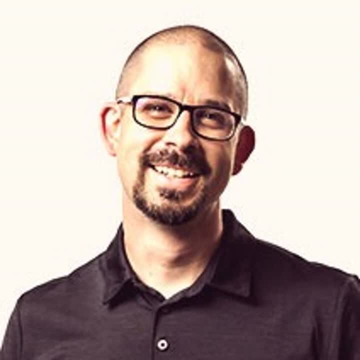 CodeQL has to manage all of that. It does, It does, Indeed, And we have. we have an amazing team who is building, essentially, language models for each one of the languages we support and continue to evolve them, And it's not just a once and done. 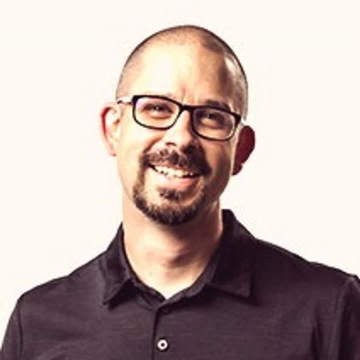 build either, because, as you know, these languages evolve all the time. There's new releases, there's new versions of Python coming out, you know, constantly, And so how do we keep up with that? I think there's there's kind of two angles here. One is: how does the team continue to model? 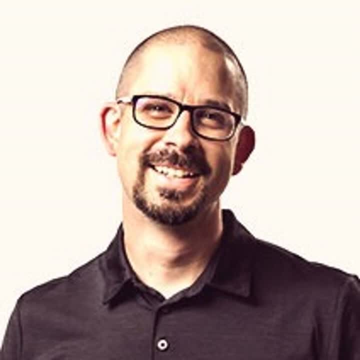 and create what is considered a vulnerability. We approach this a few different ways. One is we actually have researchers inside of GitHub who are doing vulnerability research on open source projects and they're actually actively contributing what they're learning back into the CodeQL base, which then is then made available to all of our customers and open source. 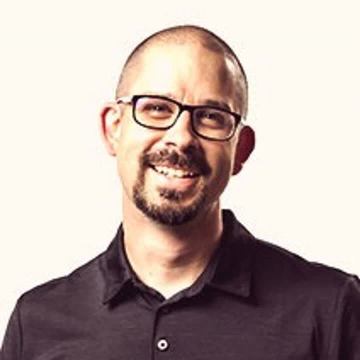 users, typical devs all the way to, you know, big enterprises. And then we have started to use AI to help auto model languages faster and open source projects that are widely used, so that we can actually increase the rate that we are. 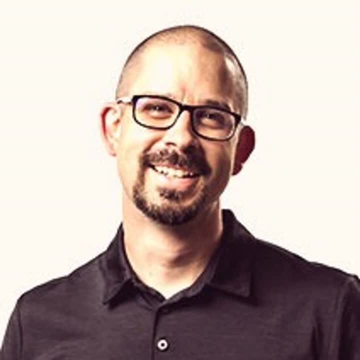 are modeling and supporting new capabilities in that program. Now I was picking random languages, but I do want to come in to give a brief, brief correction. I ran, I called out Rust and Erlang, which are you know. I thought about. 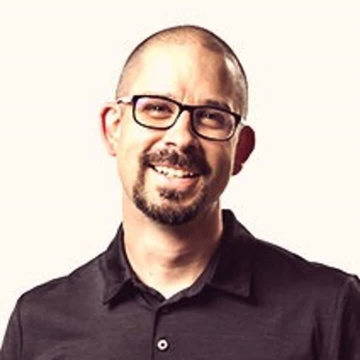 them a little bit more on the far side of the bell curve there, but those are not supported. You have C, C++, C, Sharp, Go, Kotlin is in beta. You've got Swift in beta, which is pretty cool, Python, Ruby. you know what I'm struck by with this list is you've got both compiled and 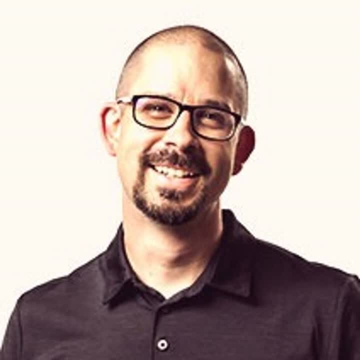 interpreted languages, which are two different universes that you're going to have to treat as if they're the same, but they're very, very different. They're really different in terms of how we approach it. The team's making some incredible progress to be able to tackle even the compiled languages in a faster and I'll just say like: 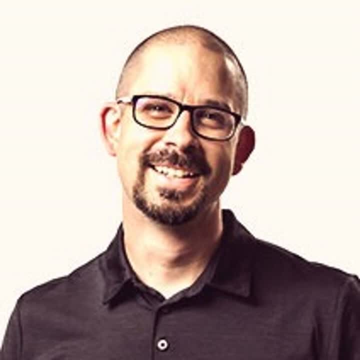 easier to set up ways, because right now you often have to like integrate it into the build, as you're thinking about like a Java build. The goal here is to really make this easy to turn on, easy to use and kind of easy to get to that first meaningful alert that moves the needle. 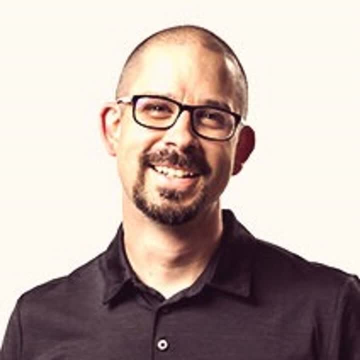 on the security here And they're making a ton of progress, So I'm excited to see where we're headed as a program there. The amount of like work happening to just push a hello world like the back, the behind the scenes work, must be insane. You were talking about free compute. Like if I go and make helloc and I check it in, for me it happens instantly. I see the file, I can set up a GitHub actions, I can make a release executable pops out and then I can start hitting raw dot, whatever, whatever, and I can start dropping, I can curl it immediately. 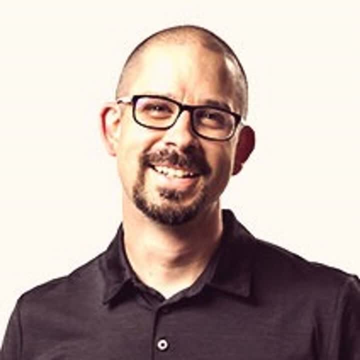 But behind the scenes, you've run CodeCure, you've scanned for viruses, like there's a whole bunch of compute that happened And you did that on a public repository. Is this going to be sustainable? You just make it more efficient. 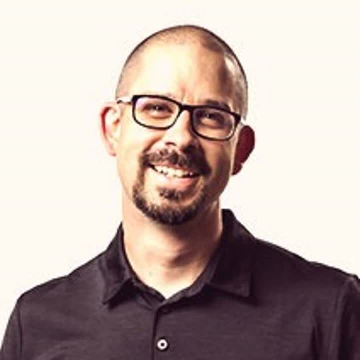 I don't understand how that's going to be something that'll be around in 10 years, but it needs to be. It's a good question. I think some of it's about the efficiency And I think some of it is about the fact- and this is one of the things I love about GitHub- is that you know the leadership. 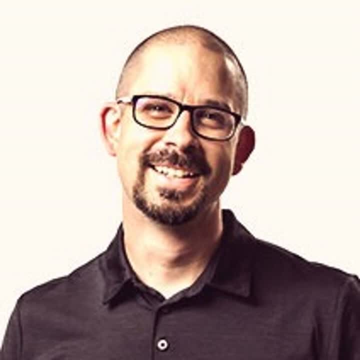 and the company generally values this community and values the work we're doing here and is investing in that as well. And so I think you know it's not necessarily a question of like: can we make this cheaper to run or not for public repos. It's like: how do we do it? Is it scalable at all? You know, 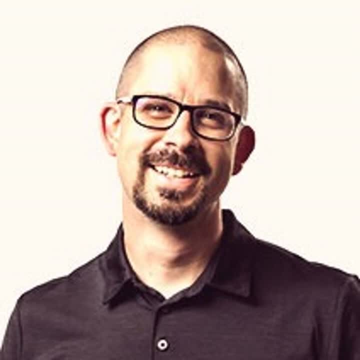 period for some of the capabilities, And I think it gets a little harder when you talk about GPU bound AI features. But generally you know it's an important part of what we're doing as a company and as a business to support the open source community and continue to lean into. 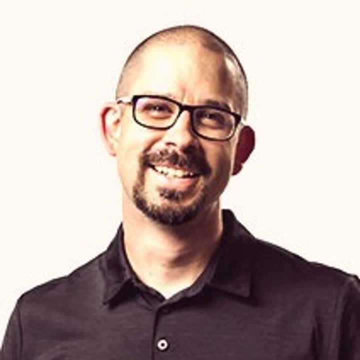 that responsibility So kind of over all of this. like looming over all of this is GitHub Copilot, which is generating code. there's a large language model at its base, But large language models are tuned for different stuff. Some are good at generating Shakespeare and limericks and some 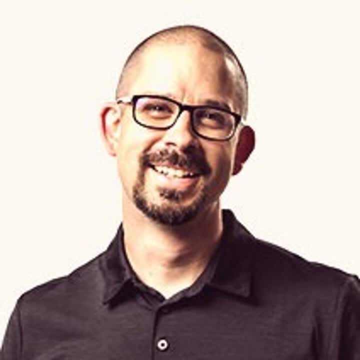 are good at generating code, But some are just confident BSers. How do I know that Copilot or some code language model is not going to go and generate insecure code and then run it down my pipeline, my security pipeline, Sure, So kind of starting at the left side of this, the models we're using are very much focused. 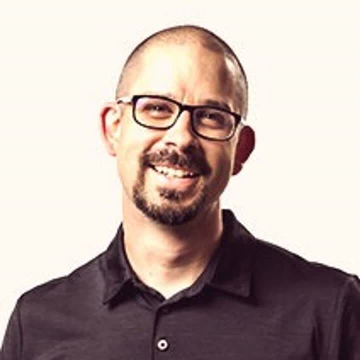 and tuned towards Software development and the way we're incorporating those, And so we're going to continue to work on what's the right models to use for the right situations here, And that will evolve as the product evolves as well. But then kind of, if you move a little bit to the right, 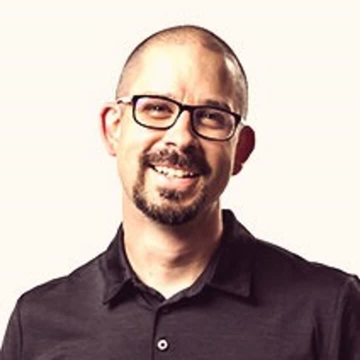 then we are working with Microsoft and we've got our own filters in place as well, that we've partnered with Microsoft on. that do things like security filtering and toxicity filtering. So they're looking for common MySQL injection vulnerabilities and are going to prevent those from even being suggested to developers before they even get there. Now, this is early. 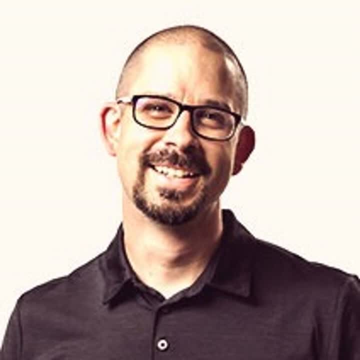 days And I think this is going to continue to evolve And I'm really excited actually to see, over time, if we see fewer and fewer vulnerabilities introduced in the editor. to begin with, because I actually think we are. We're already seeing that now, But you know, I think getting these filters 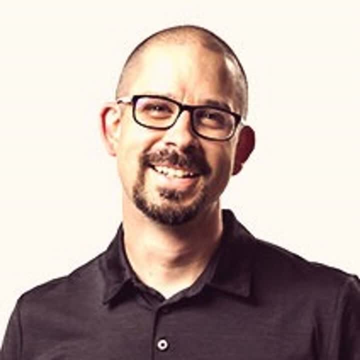 getting the tuning necessary after the suggestions to make sure it's relevant to the context of what the developer is doing. what they're trying to do, what question they asked, is something we're very focused on And I think that's going to be a really important part of the development. 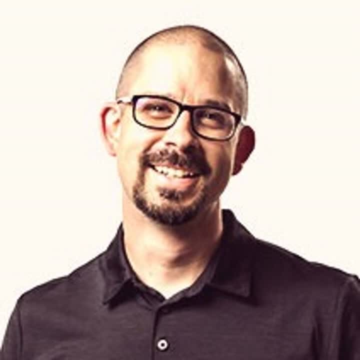 And then you know, we always say, even though these suggestions are good and we're seeing huge acceptance rates here, it's a co-pilot. So you should still run advanced security, You should still check the code, You should still make sure your builds work and do all your normal tests. 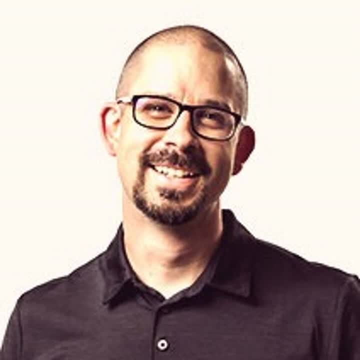 as you would normally. I appreciate the call out about the idea of context. I use that in my talks about not just co-pilot but AI in general. is that if you walk up to someone and you say that they're going to like- I joke about this- my wife and I we finish each other's sandwiches, You know. 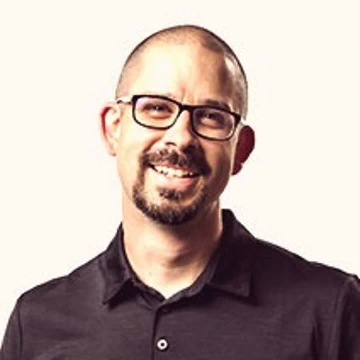 that's like maybe it's context that we have because we've been married for 25 years. But when you say to GitHub co-pilot, Hey, write me a for loop, How much context is appropriate? Does it need to know what I wrote last week? Does it need to know what I wrote earlier today? 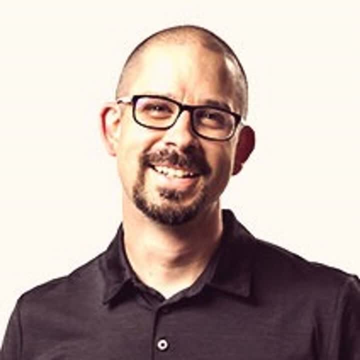 Or can it produce what I need it to produce now. Maybe it doesn't know that I'm in the middle of red teaming, or maybe it doesn't know I'm in the middle of whatever context that GitHub co-pilot knows can get into an uncanny Valley of creepiness where I might feel uncomfortable that the AI knows. 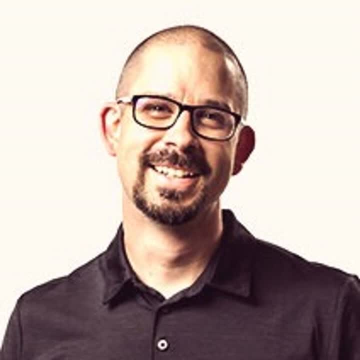 But if it's permissive and it says follow up questions like I don't know, not like clippy, but you know what I mean. Like looks like you're doing some naughty things with red teaming- Would you like help Versus? it looks like you're really focused on security and you want your code to be. 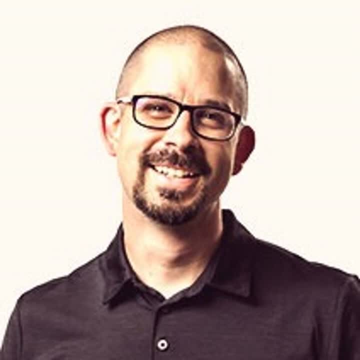 extra secure. How much context should co-pilot have when it's trying to help me? Sure, I think you know this is something we talk to customers about, And I know our product and engineering teams are really focused on as well, And I think some of this is going to come. 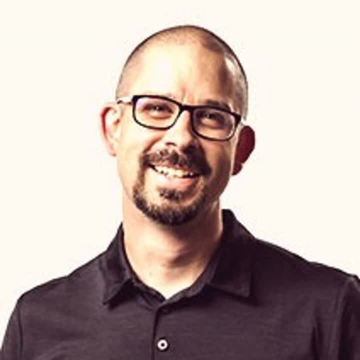 down to where in the product and where in the workflow That the developers engaging AI as it is, And so you know the context. going into co-pilot, GitHub co-pilot- from auto completion, maybe open files in the editor that they're working on now. But if 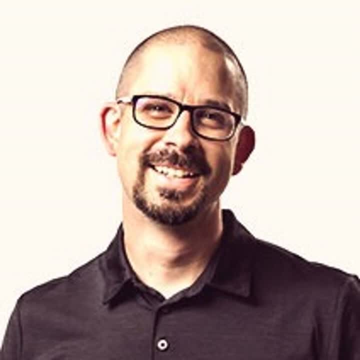 they've got chat- GitHub co-pilot chat up as well And they're asking questions. then that can tune and help it understand a bit more. And so as we kind of are building GitHub co-pilot into more and more of the GitHub platform in terms of enabling developer productivity and end, I think. 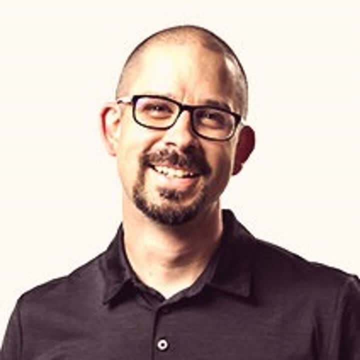 we see that be more evident to developers where it's getting it and how it's helping them be more productive. I like that, the evident part, like I don't want magic, I want code, QL or dependent bot or any. 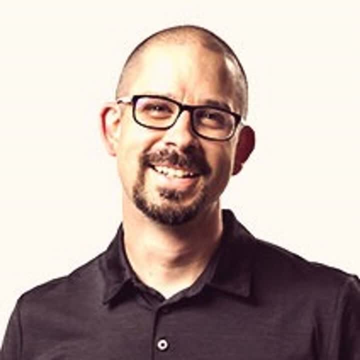 number of these tools and GitHub, advanced security and my pipeline to let me know: hey, I found a thing, Here's why I think it's a thing And here's what I think you should do about it. Like, don't just say this is a problem. Tell me why you figured it out, So then I can learn and be better. 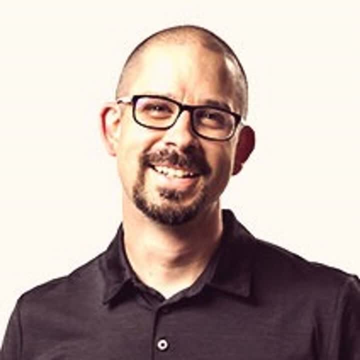 myself. Sure, Yeah, no, I totally agree, And I think you know when I will pull up co-pilot chat and start asking questions. that's one of my favorite parts about it actually is it's explaining to me here's. 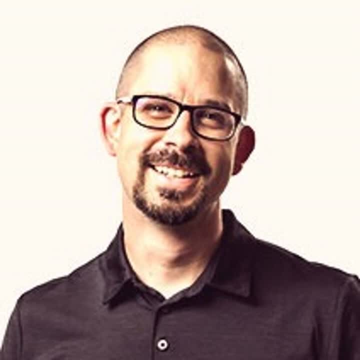 what we're suggesting. Here's why, hey, this is vulnerable. Hey, if you want to read more about why it's vulnerable, go click this link And it just honestly, it's a much richer experience than going to a search engine and trying to find help for the thing I'm trying to do, And it's also 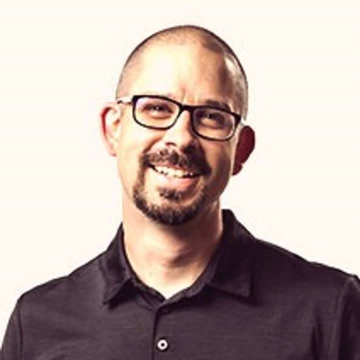 way, way faster. I was editing a Jupyter notebook the other day to like analyze some data for the teams And I needed to make some changes to it And I wasn't super familiar with the language And I was like, oh, this is going to take me hours, I'm not even going to bother with this. And I was like: 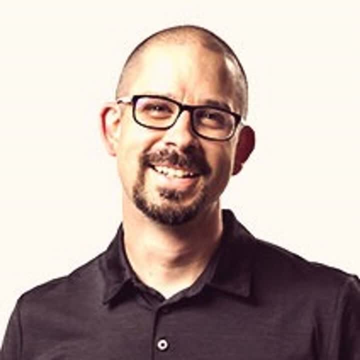 oh wait, actually let me fire up co-pilot and see what I can do. I had it fixed in like five minutes. It did exactly what I wanted it to do And I understand why it did it, And that was just. 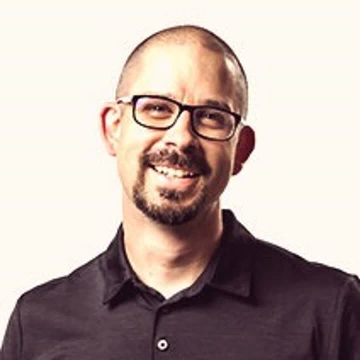 a fun thing for me, given that I don't really develop every day anymore in my day job, You know. it's interesting that you call that out though, because you know that idea that there are co-workers or relatives who are really good Googlers. You know, I'll have like non-technical 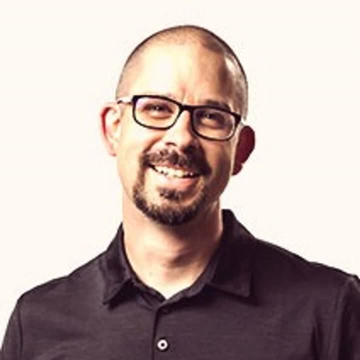 relative try to Google for something And I'll be like, oh, I'm not going to be able to do that And they'll just keep banging their head against the wall. And then I just I'll notice like you used too many words, use less, and then I'll find it on the first try. 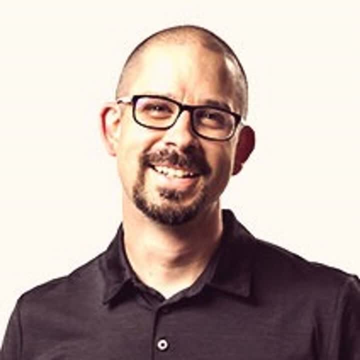 Or there's a particular term. Hopefully, co-pilot and AIs will equalize that more so that everyone will get the answer that they want. Because what happens now is my non-technical relative will be like: oh, you're just a really good Googler. It's like, well, no, you know, I want to teach you how. 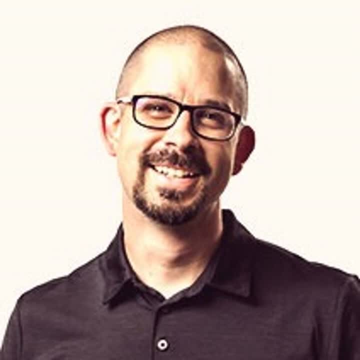 to be able to do that. But I noticed that their solution is to simply restart and try again. Yeah, Like give up on the query and or raise it differently, But with an AI or with a co-pilot. I don't just give up and start a new. 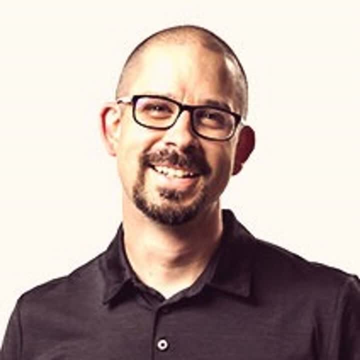 conversation. I try to refine it And I think that's a skill we're going to have to teach our non-technical brethren. I agree. I also think, at least to me- it feels more intuitive to do that with an AI co-pilot. I mean just being able to have that. 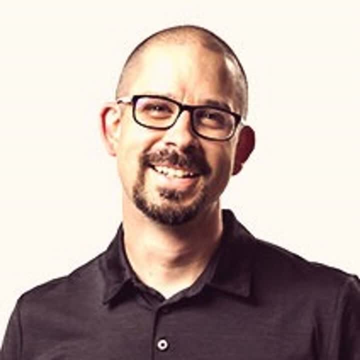 context we were talking about a few minutes ago, that it's already got it, already sort of knows roughly what I'm trying to do, or at least what I'm seeing on my screen, to a certain degree and say like hey, can you explain this file to me?